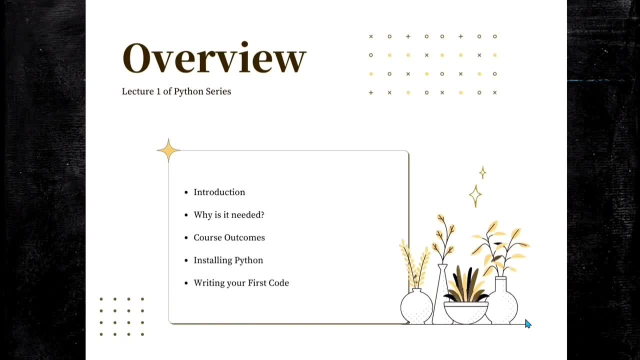 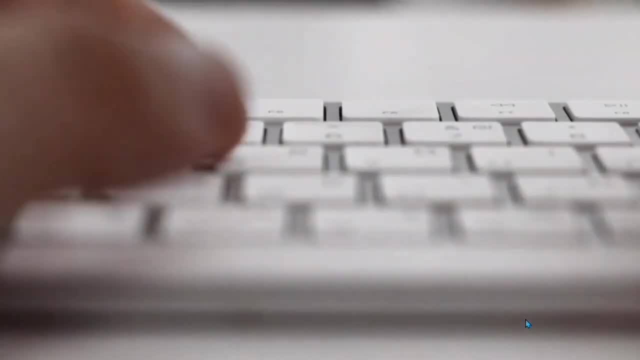 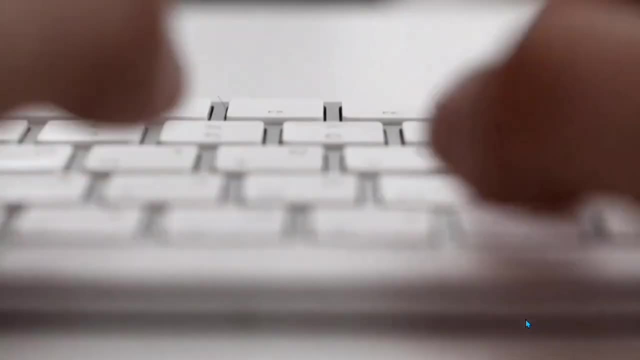 And then we will try to write our first code. So, without any delay, let's start. So coding actually has emerged as the number one in demand skill in the recent years. So whether you are going for a job, higher studies or a PhD, this is the one thing that is required almost everywhere. 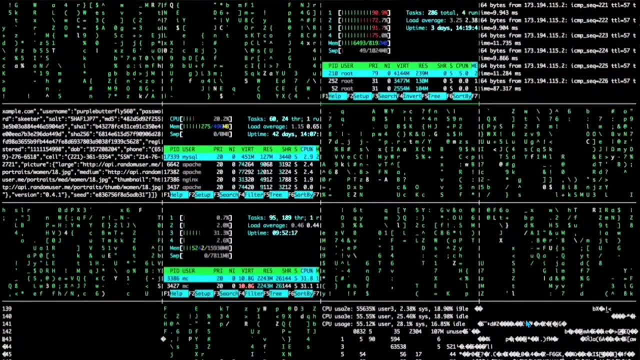 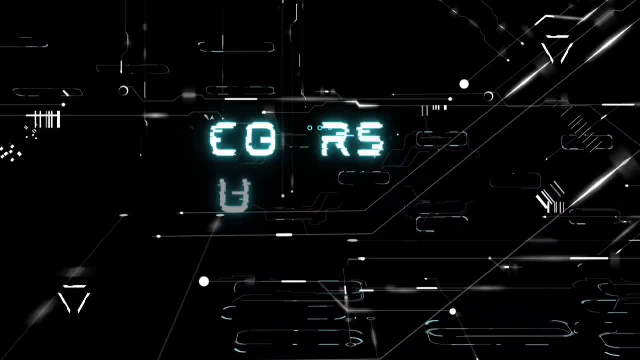 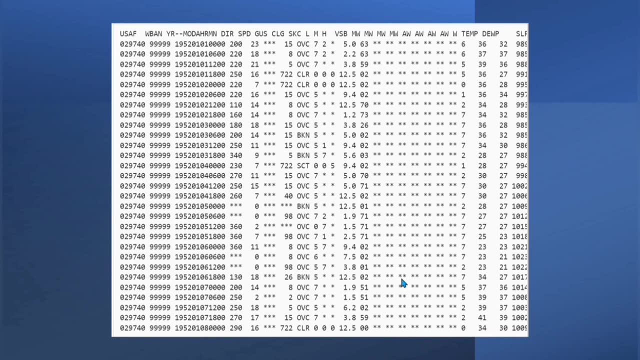 It not just reduces our time of doing things, but has also many other advantages, such as So: So one of the things we learn in this course is how to use Python to plot data. As you will know, raw data itself is not particularly useful in understanding you. 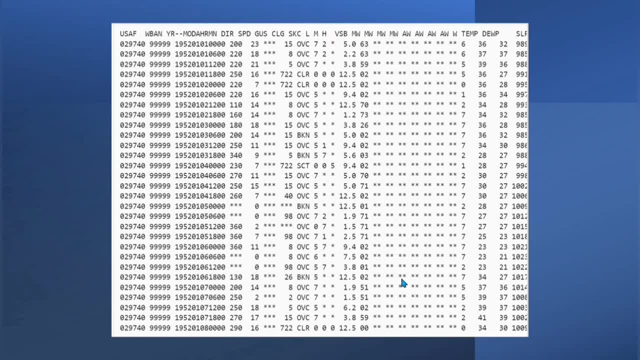 What the data shows. Let us have a look at the example that might be familiar to you. So this is a global temperature data. Now, that's exciting, right, But there's an interesting story here. We need some. We need some way to illustrate the power of this data, because this data in itself is not showing some some changes, or it's very cluttered. 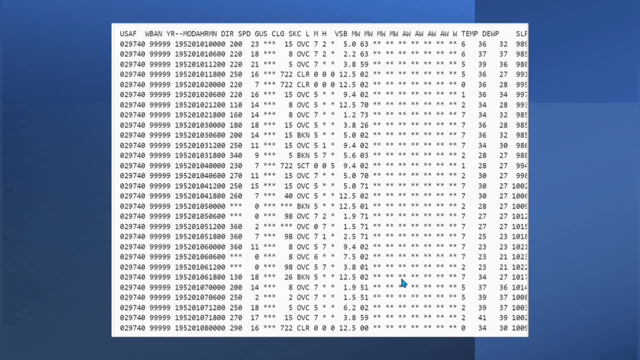 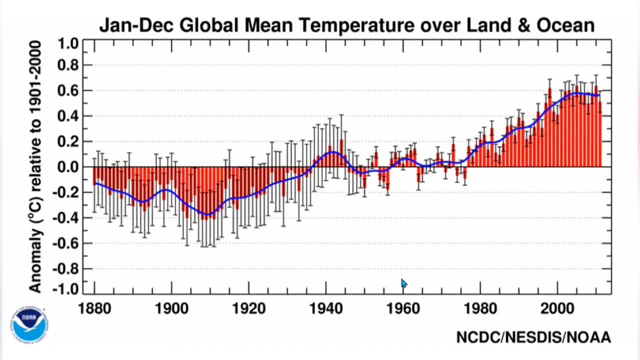 So one of the option is to use an X- Y plot of temperature anomalies versus time, And when we do that, This is how it looks. So this is obviously much better, and it is showing how temperatures have changed with time And how global temperature have increased significantly since the nineteen seventies. 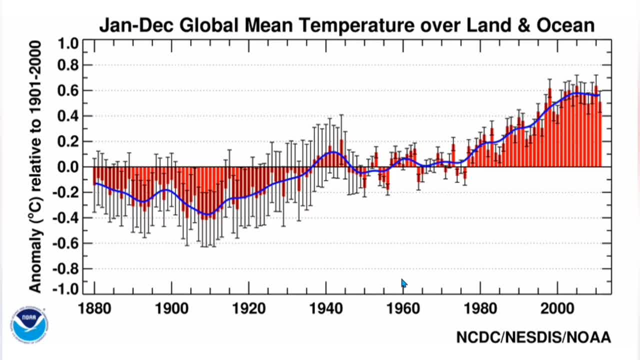 So now we see a clear step towards making data easier to understand. However, this is global data and we are missing something important about this data, That is, its connection to the geographical locations. OK, so we want to see what is the variation of this data geographically. 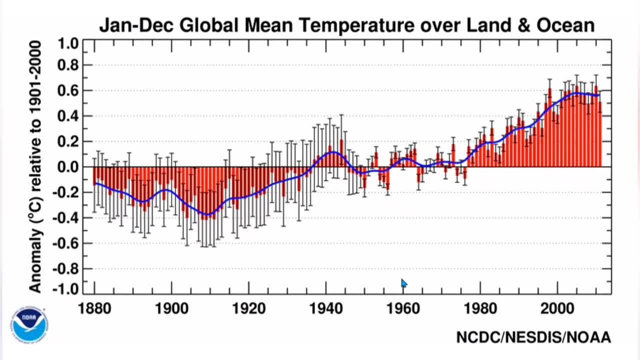 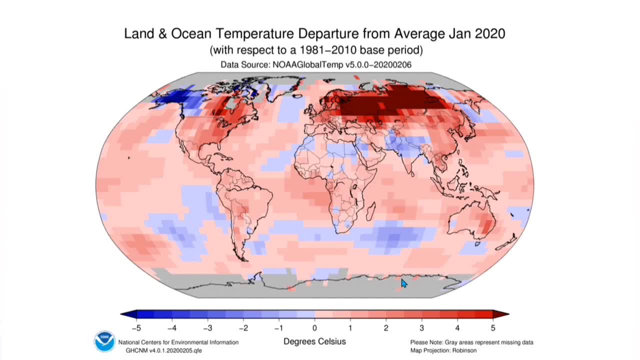 So Let us consider another option. Let us plot this temperature anomalies on a map, and then this is how it looks. Again, this helps us understand the data further, and here not only we see the change temperature, but now we also see how the temperatures vary across the globe. 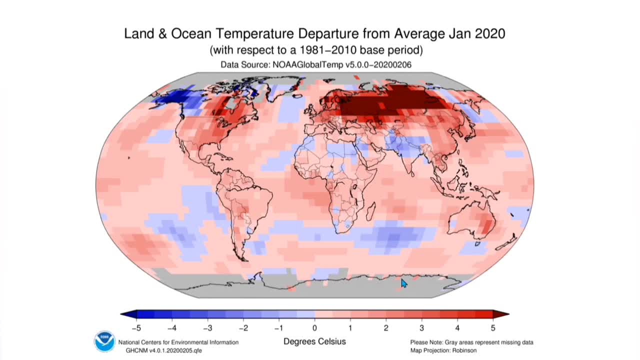 Again, the drawback here is that we only see a single time snapshot rather than a time series, So to see both it will require a truly remarkable visualization. Therefore, let's have a look at some excellent examples of data visualization with Python. So we have essentially the same data plotted above, but now we can see how temperatures vary in space. 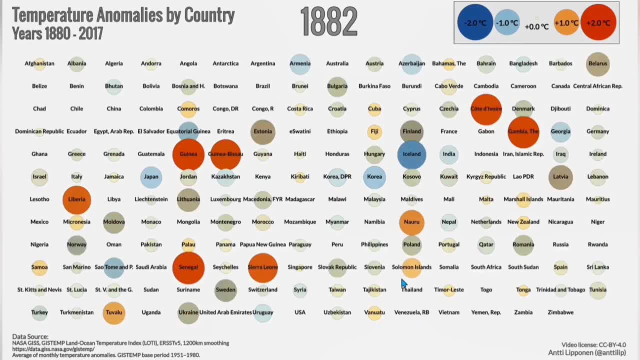 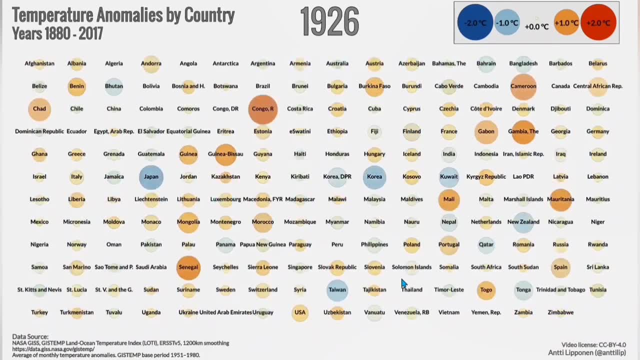 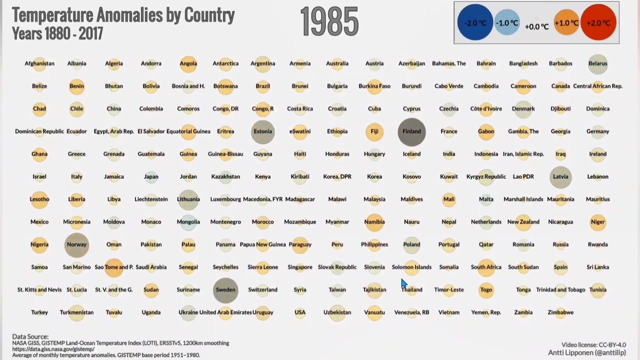 So see this. This animated plot of temperature anomalies conveys a huge information in the simplest form. people can immediately understand what is plotted, and the combination of the plot format, colors and animations are very effective. and what's even better is the fact that this animation itself was made using Python. 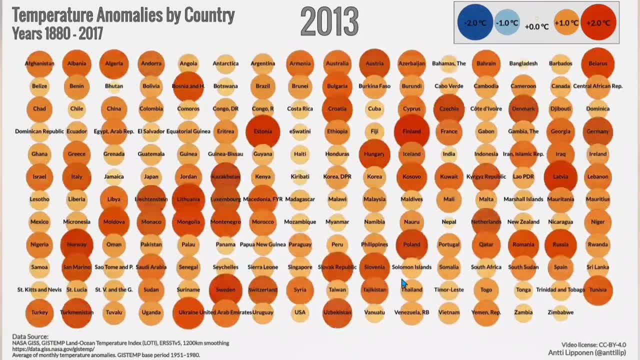 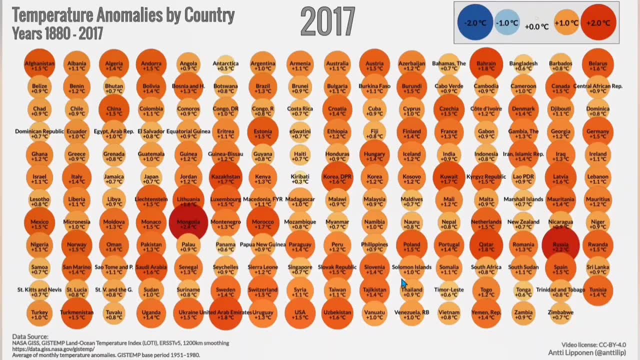 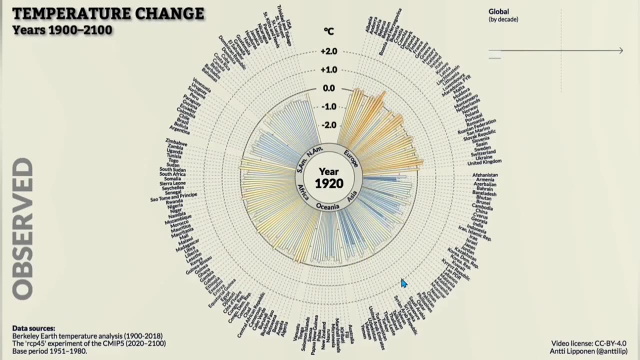 OK, another simple example of the similar data Can be: if we are able to predict the future using the given data, then if we do that, this is how it will look Now. this plot nicely conveys the warming of different regions on the Earth, again in a very intuitive form, and for the rest of the part of this course, plots like that can be our inspiration. 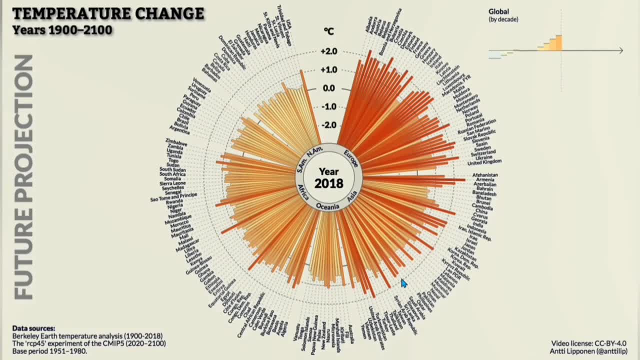 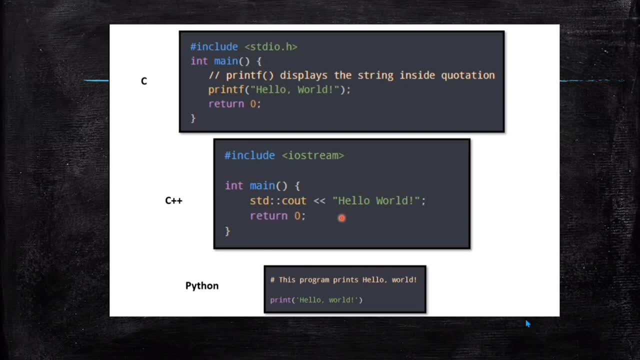 So in this course we will be learning A lot about this. So let's continue Now again to do coding. we have various languages, then why only we choose Python? so the difference is quite visible on your screens. If we write a code to print a word in C language, we need to write this much of code, right? 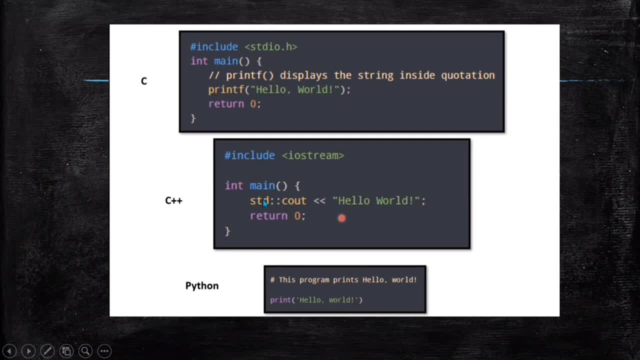 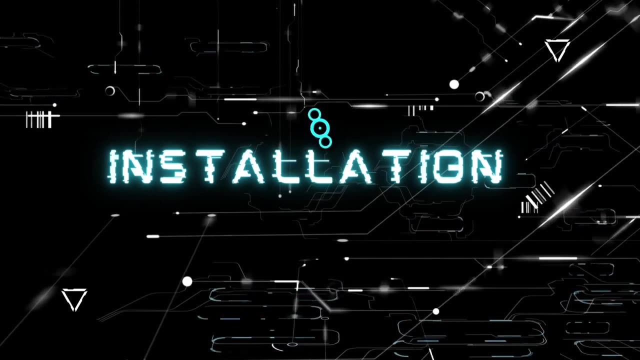 Again, if we write that thing in C++, the length is this much, but in Python it's so easy. Just Just write: print hello world and that's it. That's done. So that is the advantages of using Python. The next step in the process is installing Python. 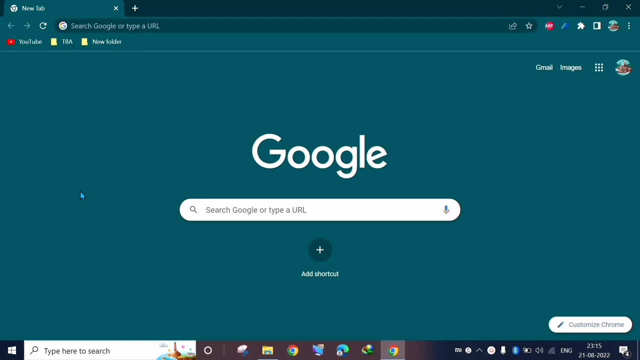 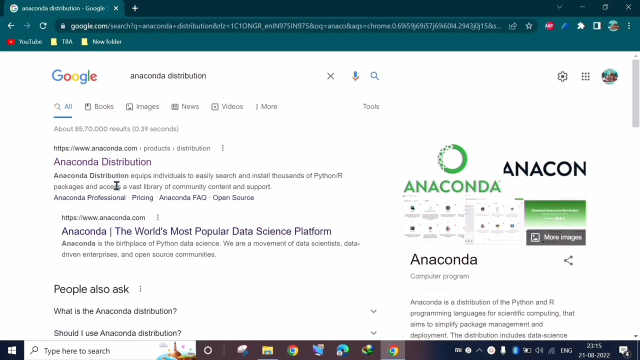 And to do that what we do is we install a free version of Python distribution system. OK, so for that you can just type Anaconda distribution on Google And once you have got the search results, what you can do is you can click on the first link and then read out the things that it shows up. 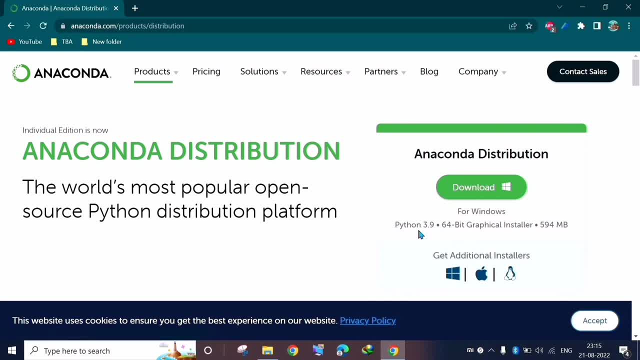 So now it shows that it is for Windows. If you are using a Mac or any other operating system, you can install according versions. So the Python that will be installed there will be Python 3.9 and it requires a 64-bit installer. 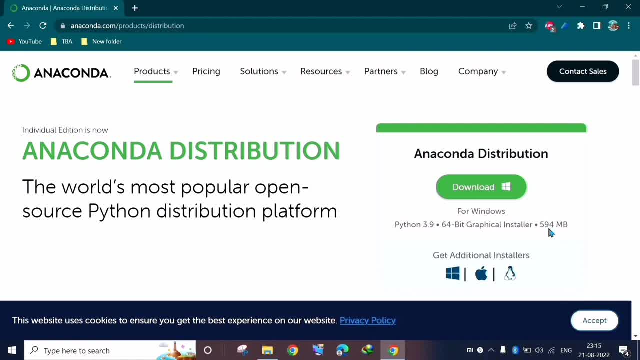 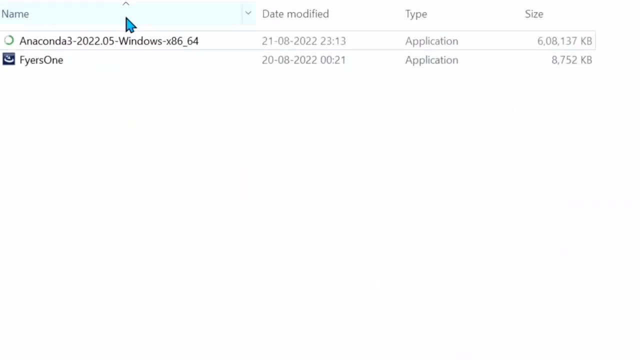 Right, Then you need at least a free space of 5.94.. But to run it more efficiently you at least need three GB of space in your computer. Now to download it, we simply click here and then the download starts. Once it has downloaded, then you can just install it. 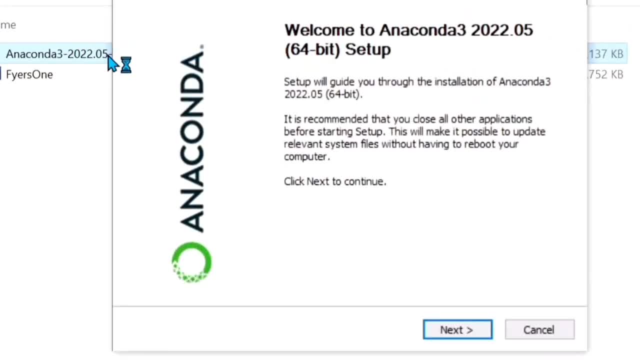 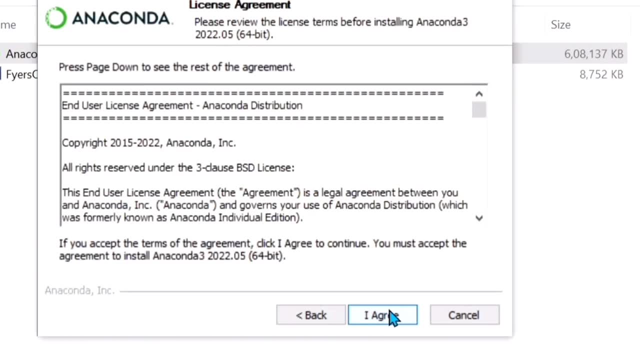 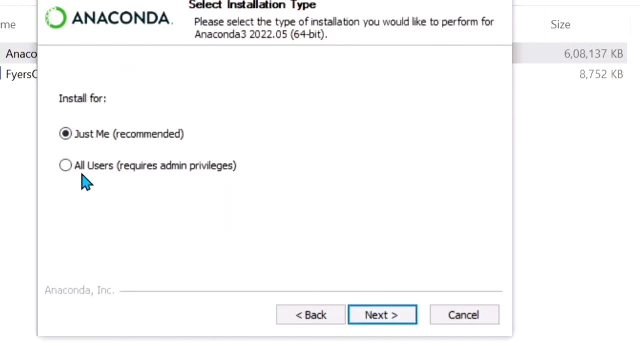 You can either double click on the folder where it is saved, or you can do this process also Now. after this, you can just click on next here. You can just read This license, if case you want to, or you can simply click on agree. 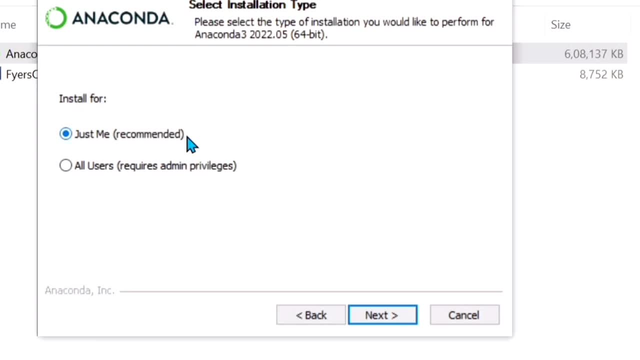 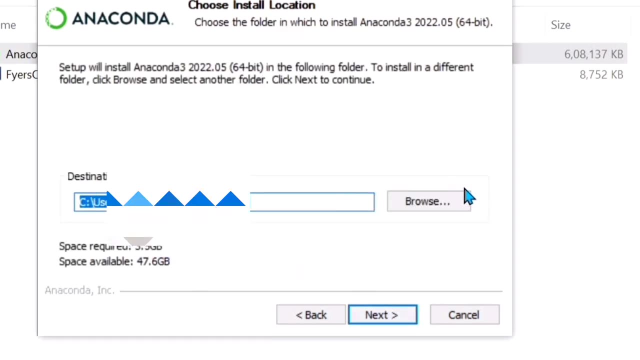 Now it is asking install, for you can leave the default setting, just me, And then click on the next button. You can see the destination folder here And, as I told you, it is asking you to have a space of at least 3.5 GB. 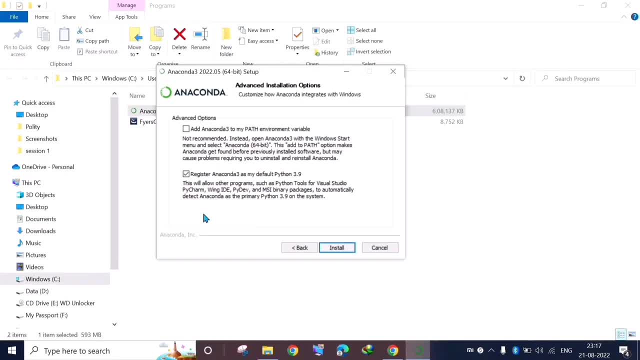 So make sure you have that Right now. after that, This is what it is It is asking. So it is asking that whether you have any other Python programs installed earlier, So in that case you can select this option so that anaconda distribution works properly. 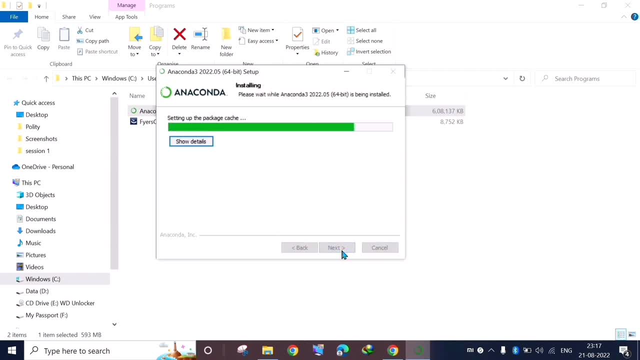 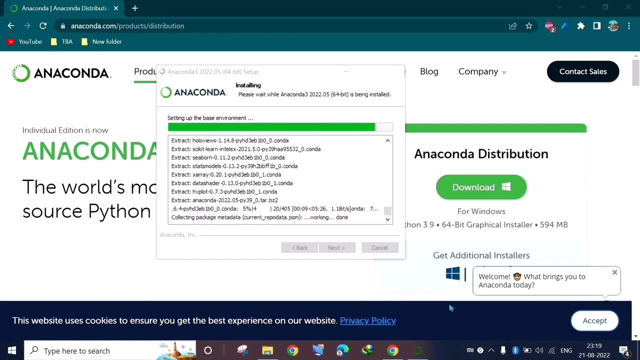 So after that you can just click on this install thing And then in a few seconds this anaconda will get installed into your computer. So we just wait for that. As you can see that it is still getting installed, So we gave a couple of more minutes to it. 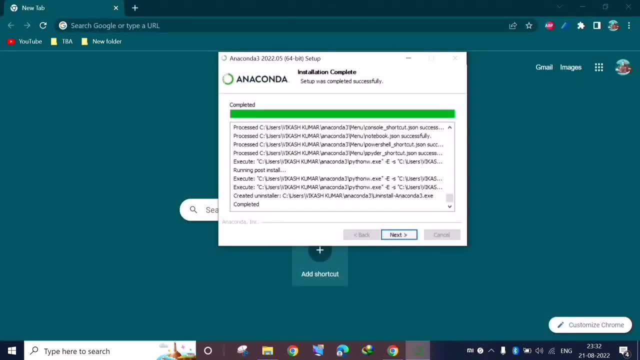 Depending on the speed or the processor of your system. it might take you a few seconds to a few minutes for this installation to get complete, And once it gets completed, you will be visiting this type of screen. Now you can just click on this. 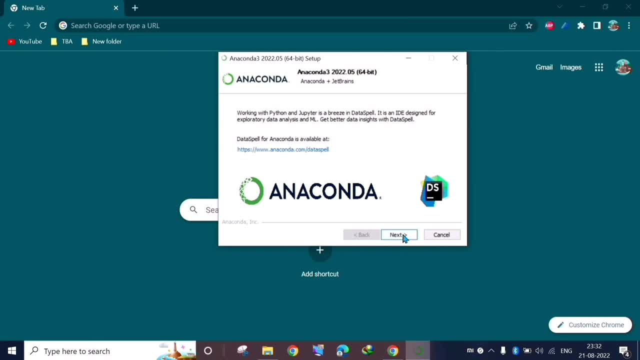 Click on the next button and it is asking you to install another integrated development environment, which is not needed for right now, because for all the things that we need to do, That much is enough. so we don't need to install this right now. so we just click on next. 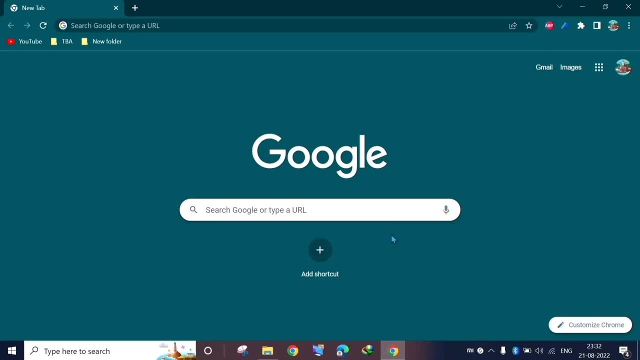 And then we finish up right. so once we have finished installing This- it might take you to some websites, but you can just cross it out- And once you have installed the anaconda distribution system. So now we just give a check whether the correct things will install or not. 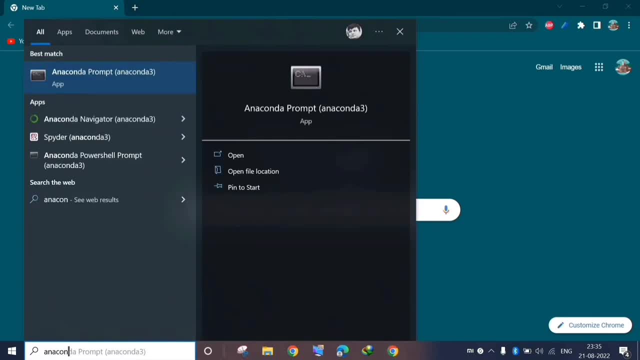 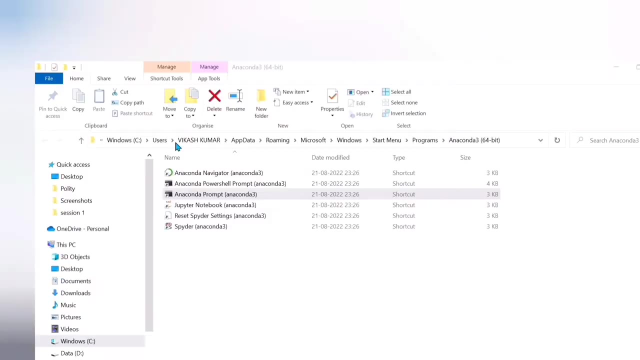 And to do that you type here: anaconda prompt, Right. So we need to run this app as an administrator. So we right click. So sometimes what will happen is the run as administrator option will not come, So you can just go on to the file location. 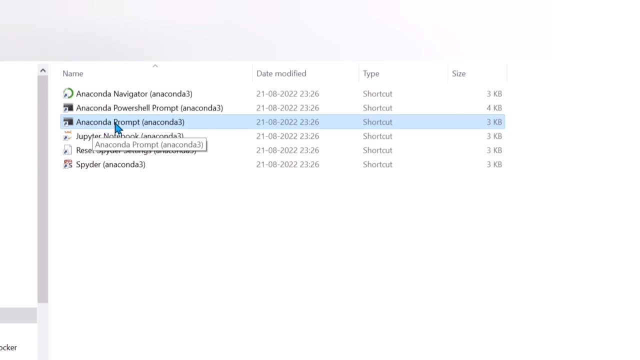 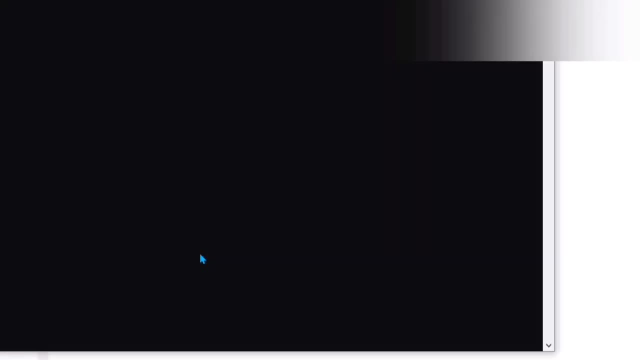 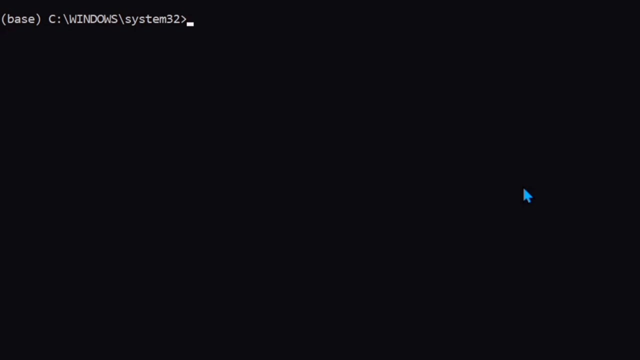 And when you go there you will see this anaconda prompt section. So now you can right click here and select run as administrator, Click on yes And then this thing comes up. So we type here: Conda, dash, Sorry, Conda. 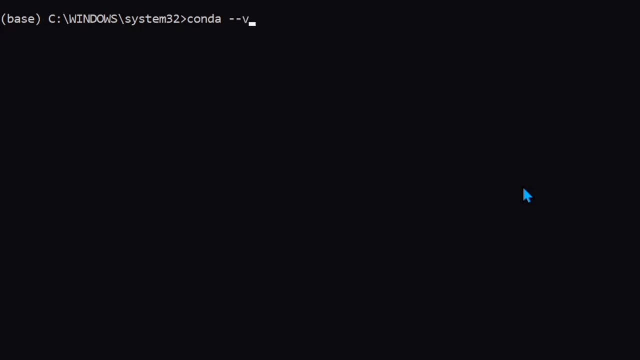 Followed by a space, Then double dash Version V-A-R-S-I-O-N, And then we select enter. So now we see it has returned that Conda 4.12.0 version is installed. It means our system has installed the correct version. 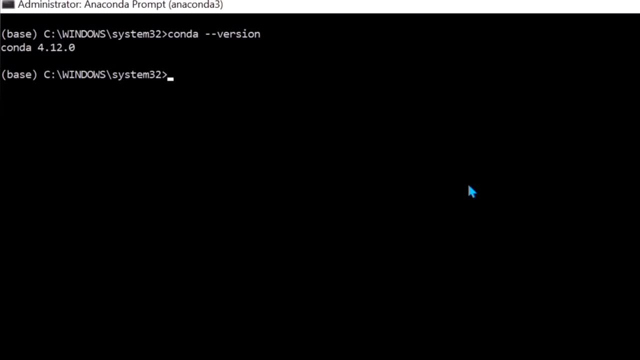 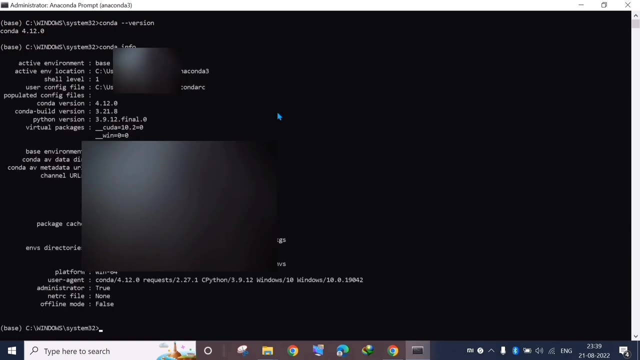 To get more information about what all things we have installed, we type the command Conda dash info and then we select enter And then this is the properties that you have installed. So you can see that the Conda version is four point one, two point zero. 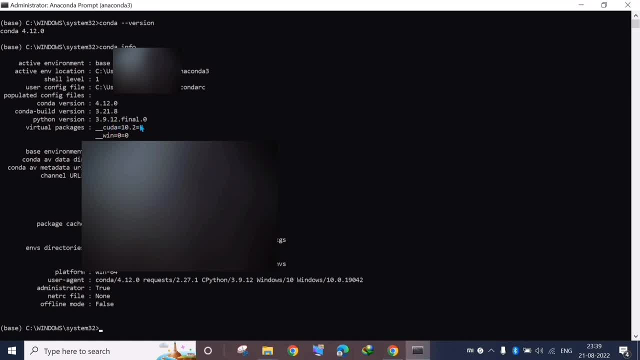 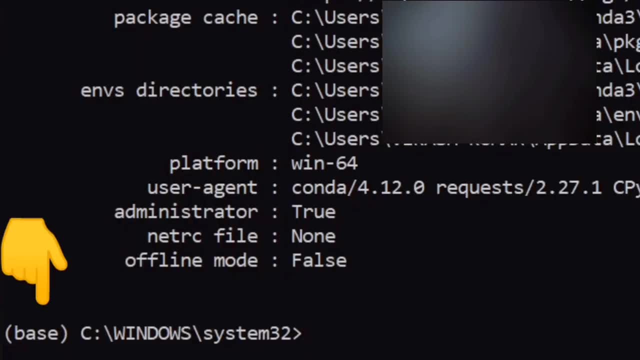 The Python version is: three point nine, point one: two dot. final dot zero. OK, so this is the environment that we are going to work on Now. you can see one thing that is written here as base, So it shows that we are working in the base environment but for our usage, at times we need to change the environment. 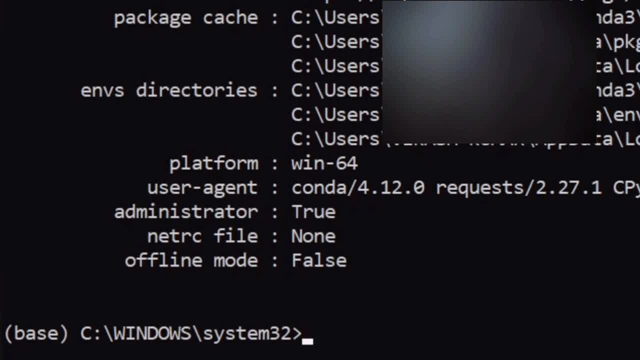 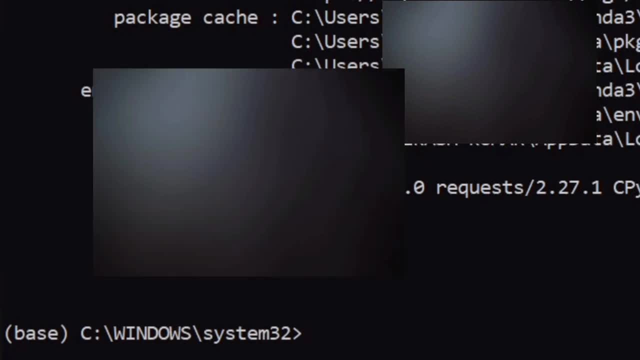 Now again, I'm saying that these things you might be finding a bit difficult because you are getting it for the first time, But after a few lectures these things will become very easy for you. So just wait for that time now to see what all packages are there. 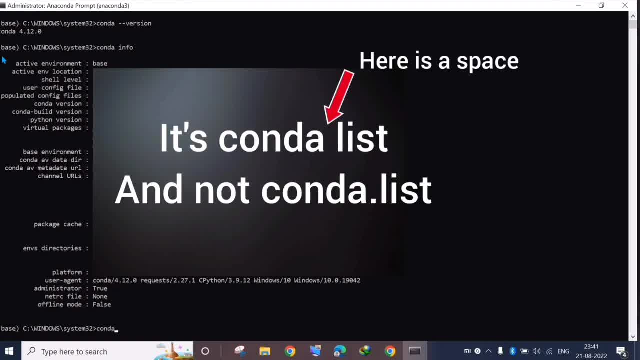 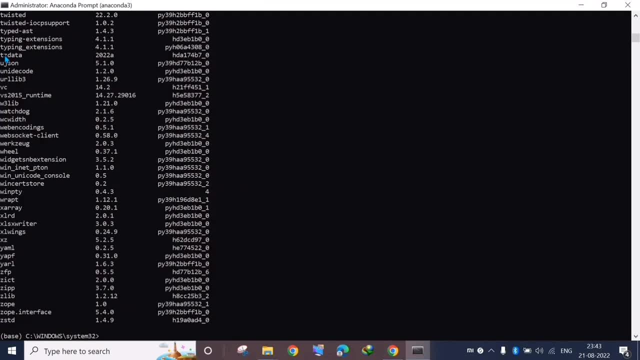 We click and type Conda dot list. Now these are the various list of packages. Now, if I want, I can explain you each and every package that is there, but that will make the lecture a hell lot boring, Right, And I don't want that. 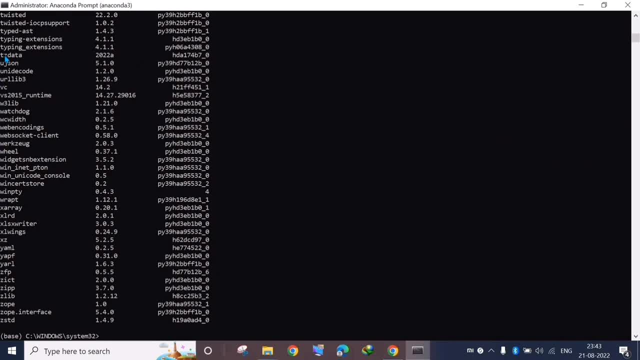 So I will teach you each and every thing when it is required to know, because if I start teaching everything then you might not get that interested in learning Python, And I want to Give things to you in a shortest possible time with utmost clarity. 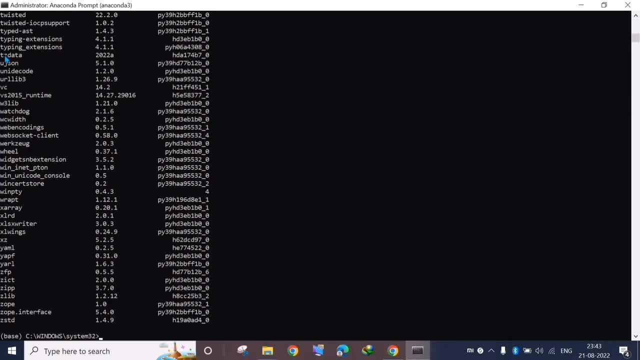 OK, so we will learn things when and wherever we encounter, and we need to use that. So currently you just know how to get a list of packages that are there, And for that I have given you a command Here. I must tell you one thing: that there 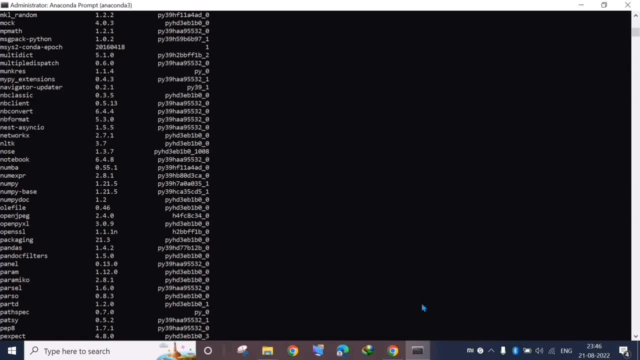 are a few packages that are not in this list and that we need in our course of this time, So that will be installed as a third party package. for example, Rasterio, GeoPanda. these all things we need to install. 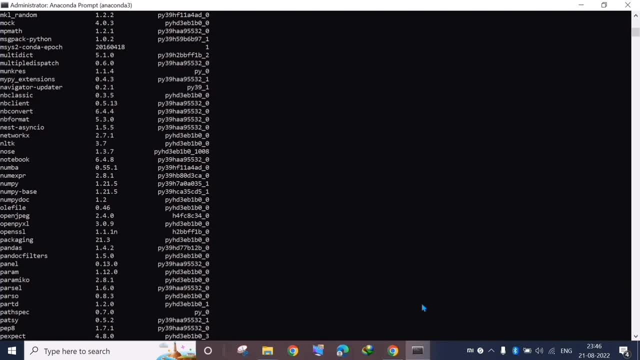 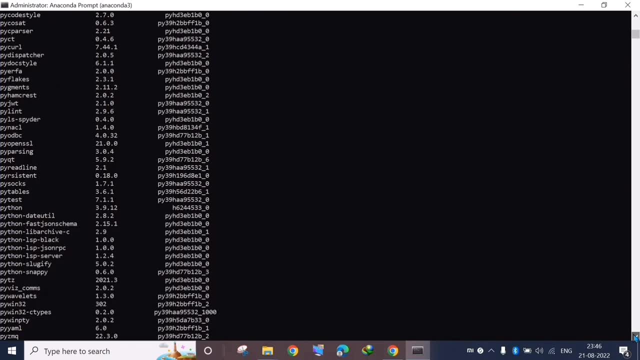 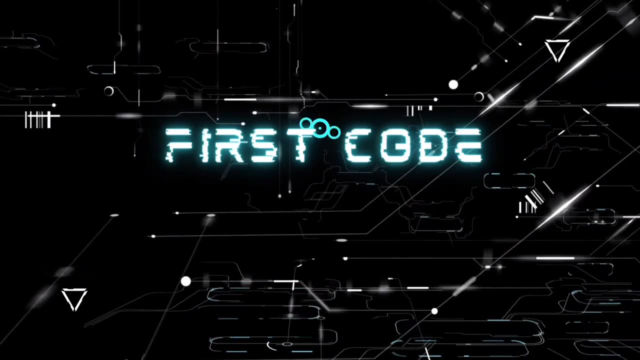 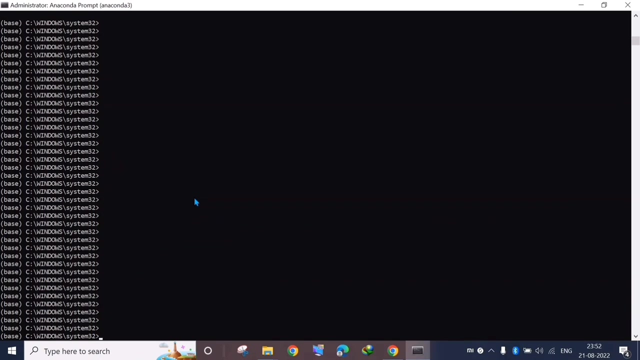 So I will let you know when and how to install and where to use it. So now, since we had a look on this package, so we scroll down and we go back to our command prompt section. So now we need to run our first program and for that we need to go to the command line interpreter system. 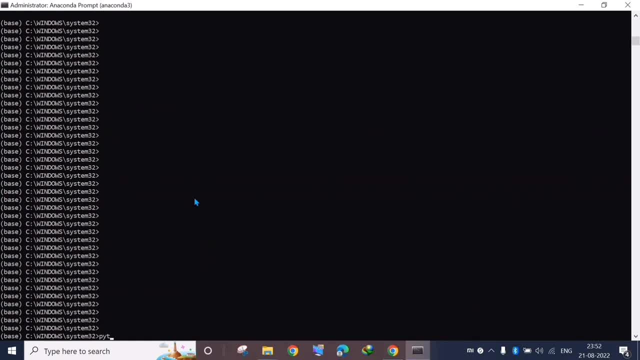 And what for a term is that? you just need to type here Python and select enter. Now you can see: earlier you were welcomed with this screen base C, Windows system 32, Python. But now you are here on a command line system. So here, whatever code you will type, it will actually run the code once you click on enter. 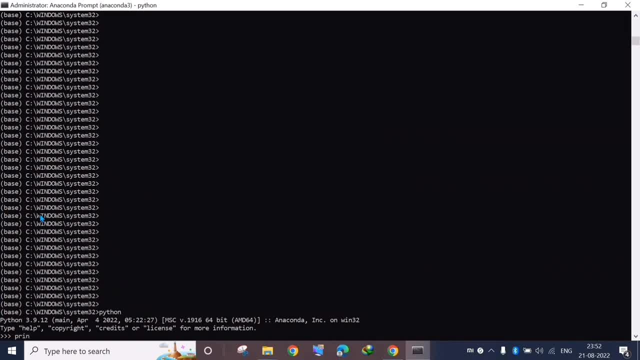 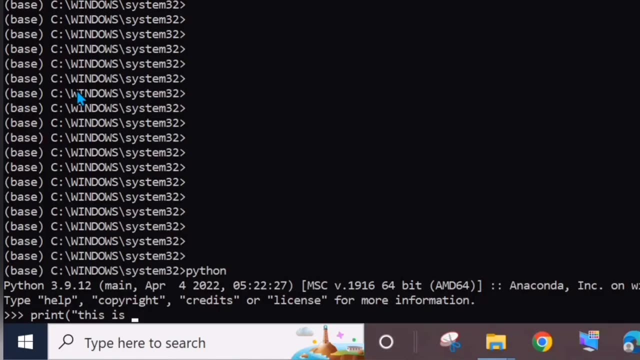 So for that we will try to write our first program so you can simply write print then in Bracket and follow. you can just type this: This is my first lecture. Okay, so now our code is complete. All We have to do is just press enter. 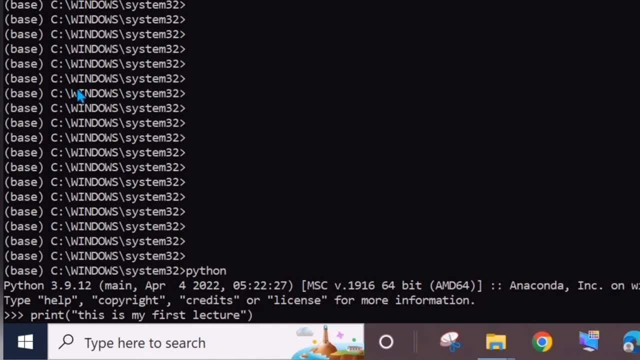 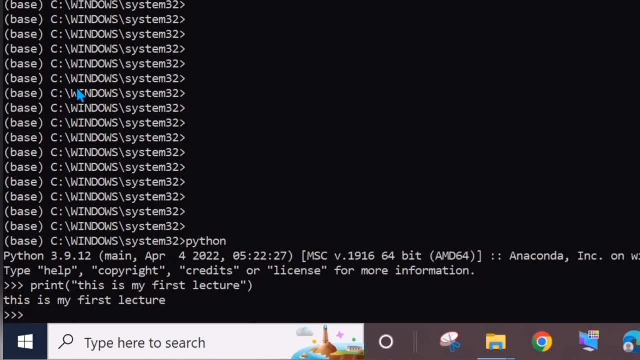 And if this gets executed it means we have learned our first program very successfully. So we click enter here and you see that your code has run OK. so if you want to switch from a Python interpreter mode to the normal mode, you can simply click exit with closed parenthesis and you will come to the base. 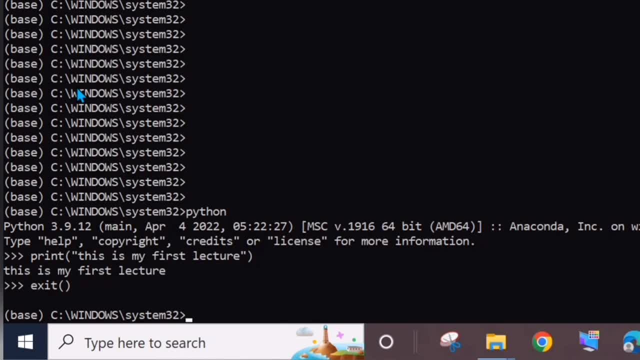 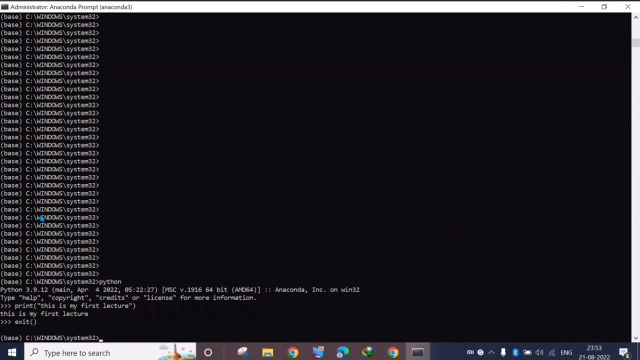 OK, so this is how simple it is. So here, Python has been installed in integration with the Anaconda distribution, but Python can also be installed as a standalone version from Pythonorg. But since we are going to use it, not as a, from a programmer's perspective, 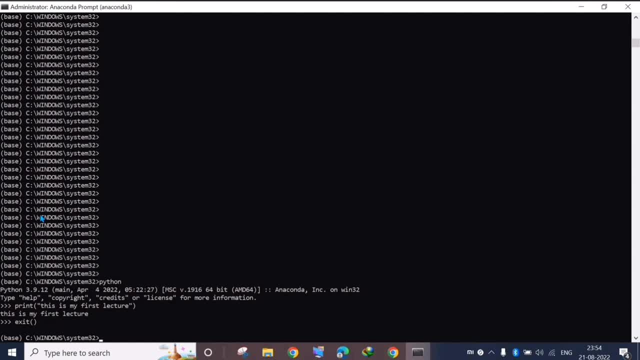 but from the perspective of a civil engineer, a water source engineer and an environmental engineers. so we don't need to go into that much of depth. OK, that's why we have chosen a relatively easier option. Now. that's all for the first introductory lecture. 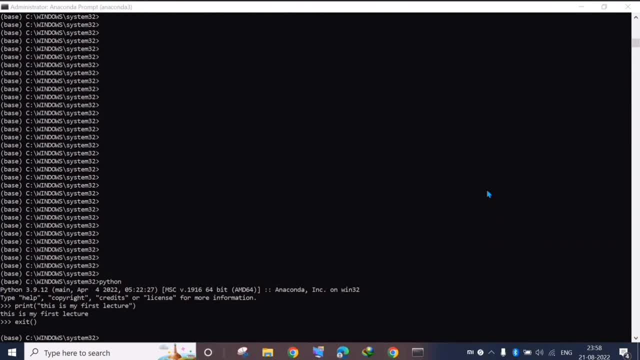 We will learn more about Python, We will learn about creating a new environment and we will also learn about Jupiter in the next videos. so I hope you like this video, If you want to get the notes And associated text, which are a little bit important.